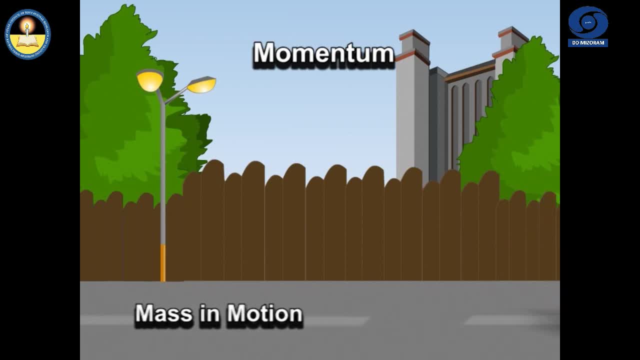 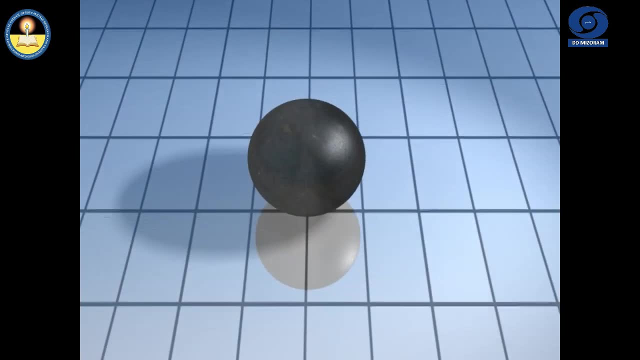 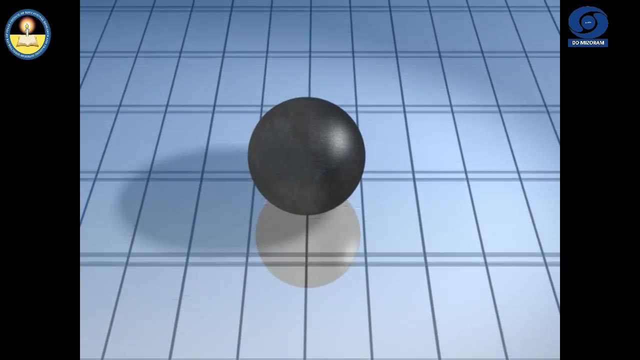 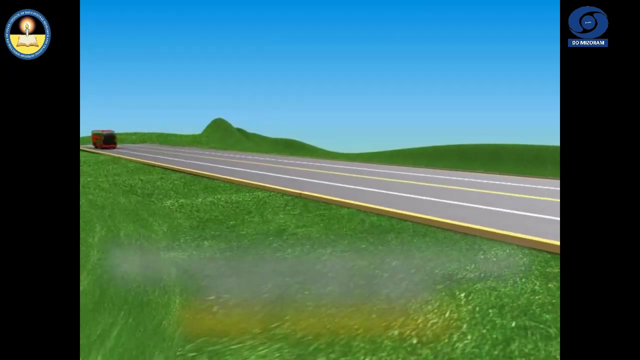 Hence, the momentum can be defined as mass in motion. It can be defined as mass in motion. It can also be defined as the tendency of an object to keep on moving with the same speed and in the same direction. Momentum associated with the linear motion is also called linear momentum. 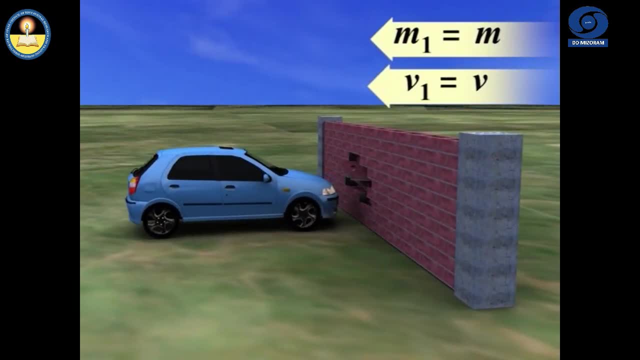 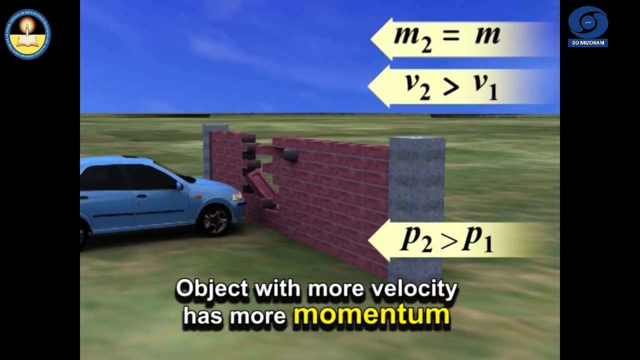 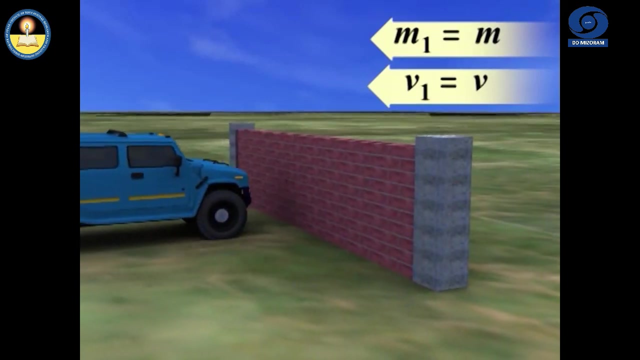 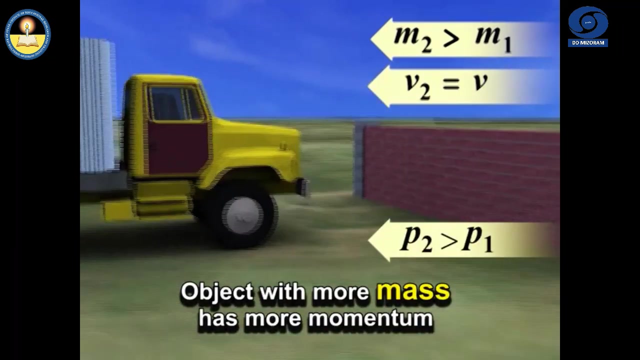 When two or more cars of equal mass are moving are moving with different velocities, then the car with more velocity has more momentum. Similarly, if two or more vehicles of unequal masses are moving with the same velocity, then the vehicle having more mass has more momentum. 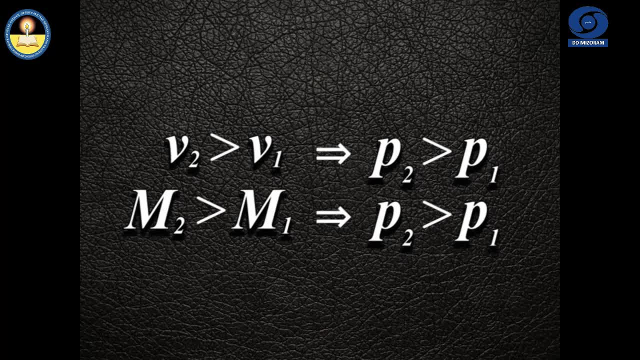 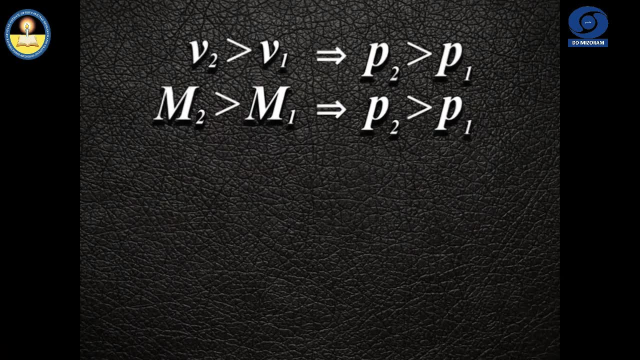 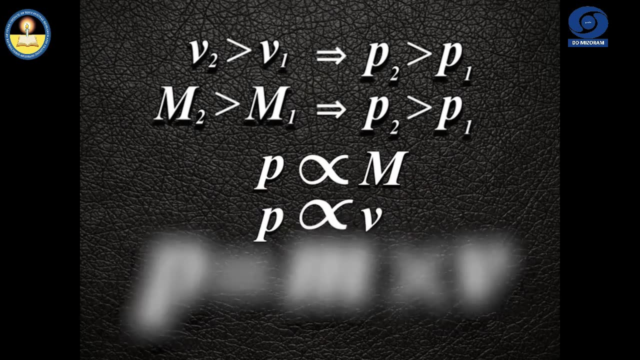 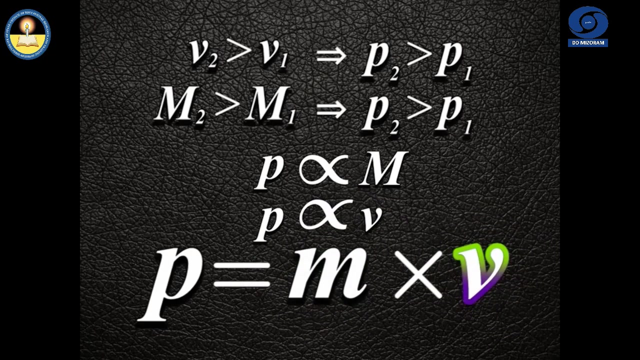 This shows that the amount of momentum that an object has depends upon two variables: How much mass is moving and how fast it is moving, Since mass is a scalar quantity and velocity is a vector quantity, therefore, momentum is a vector quantity. 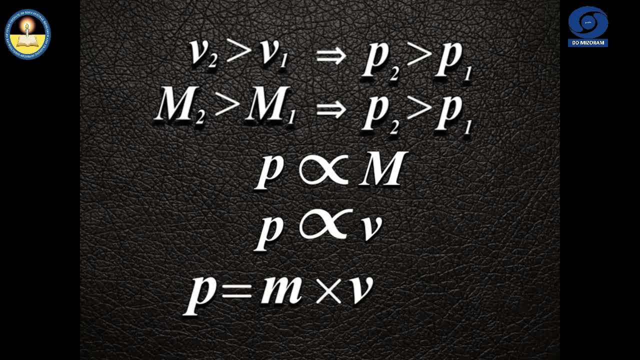 Its quantum is equal to the momentum of an object. Therefore, momentum is a vector quantity. Its quantum is equal to the momentum of an object. Therefore, the vector quantity is equal to the product of mass and its velocity, And the direction is the same as the direction of velocity. 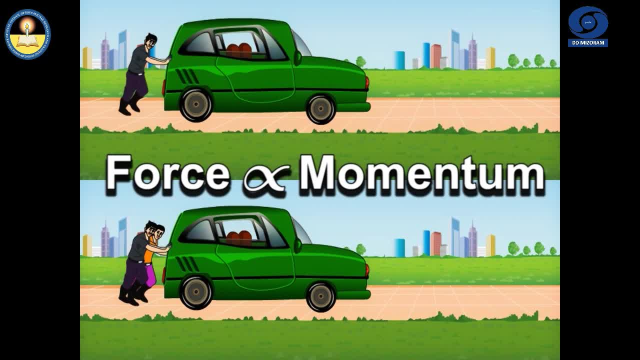 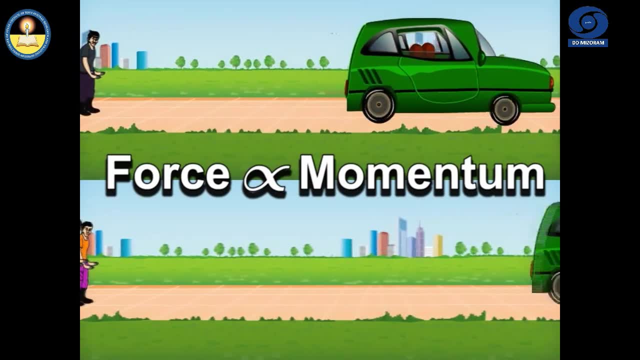 Suppose: if a force acts on a car in the same direction as its motion, then the force beats up the motion of the car and thereby its momentum. On the other hand, when the force acts on the car in the opposite direction, then the force breaks up the motion of the car in the opposite direction, which increases its momentum and increases the momentum of the car. fathers from pole. 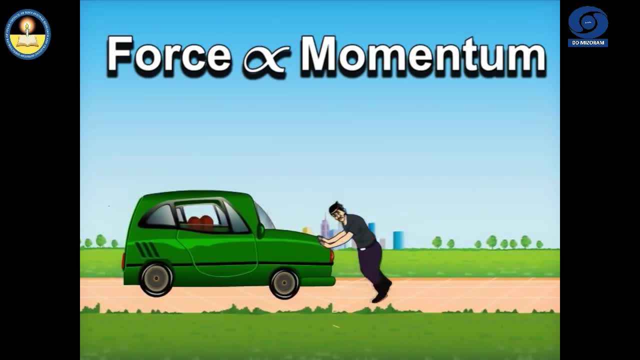 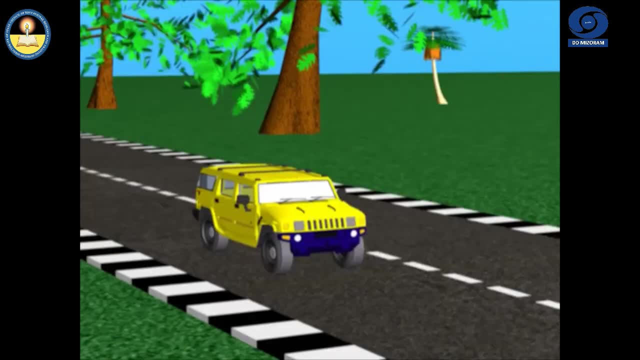 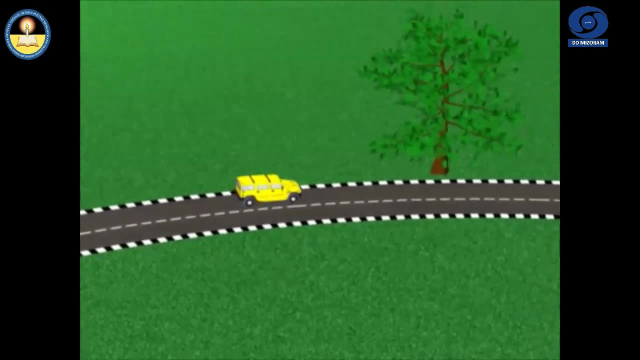 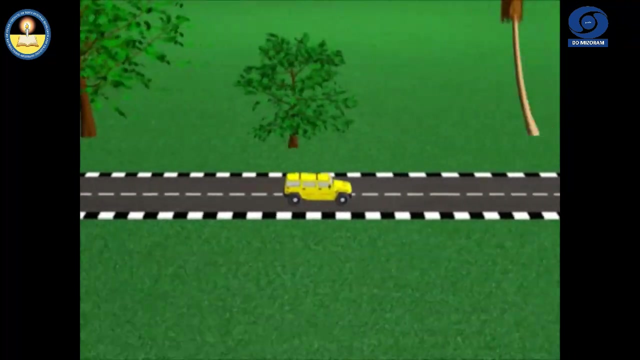 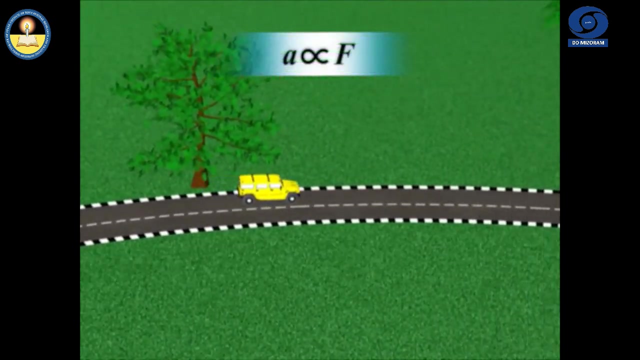 opposite direction, the force slows down the speed of the car and thereby its momentum. Know that whenever the velocity of an object changes, the motion is said to be accelerated motion. Hence, for an accelerated motion, the momentum of the object will also change, Since acceleration is caused only by the net. 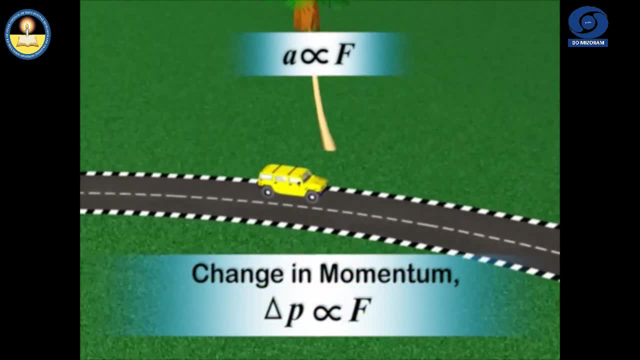 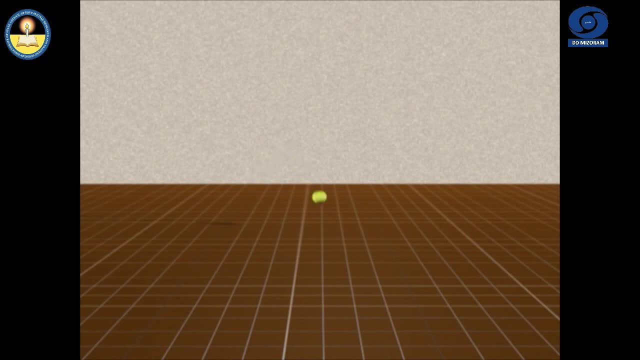 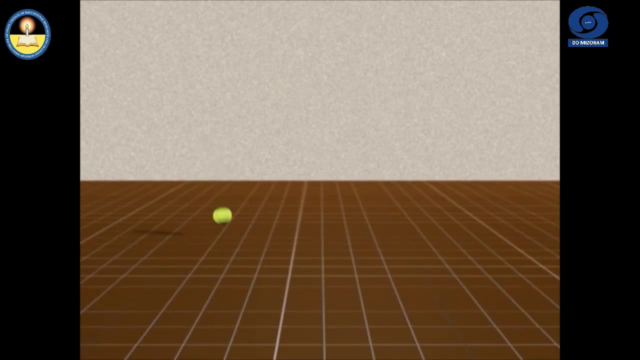 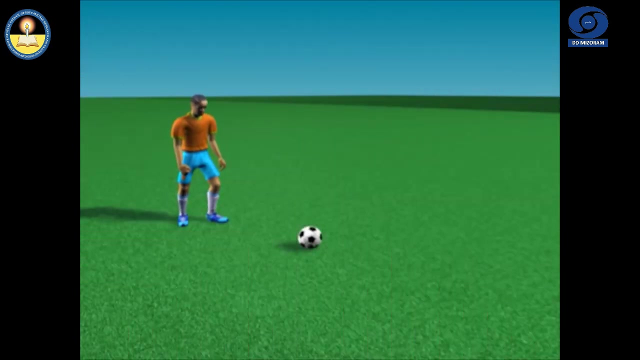 force. same is the case for the change in momentum. For example, when a ball rebounds from a hard surface, the surface exerts a very large force on the ball and there is a big change in its momentum. Similarly, when we hit a ball, we apply an unbalanced force to the ball. that produces 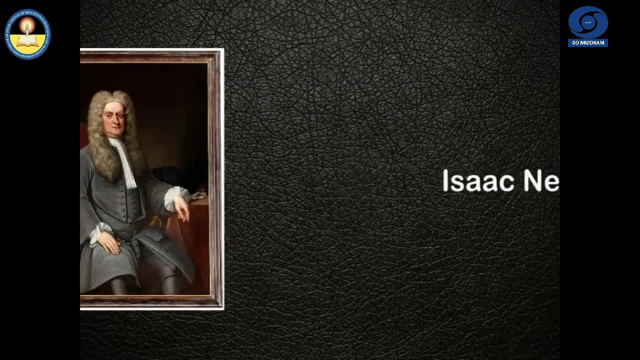 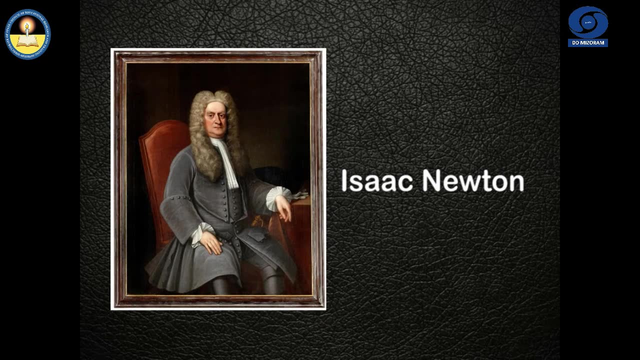 a change in its momentum. Instead of measuring the quantitative effect of force, Newton introduced the concept of momentum. According to the Newton's theorem, the set of quantities is equal to the number of points per meter, the number of points per meter and the number of points per meter. 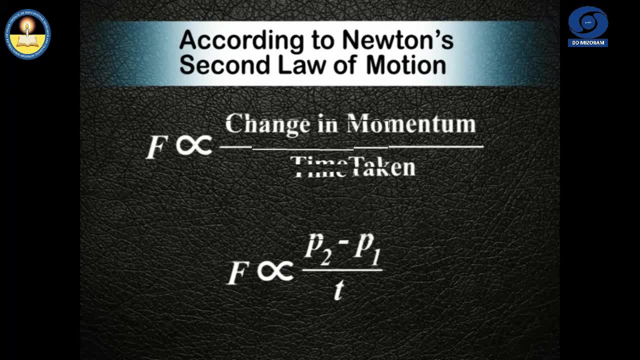 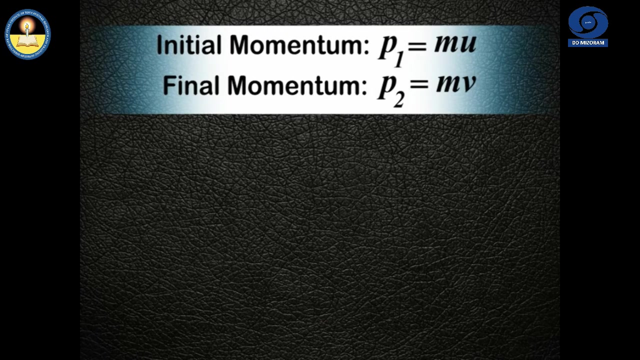 Second law of motion, the time rate of change in momentum of an object is directly proportional to the external force applied on it, and the change in momentum is in the direction of the force. If the initial and the final velocities of an object of mass m are u and v respectively, then the external force depends upon the product of mass of the object and the rate of change in the velocity of the object. 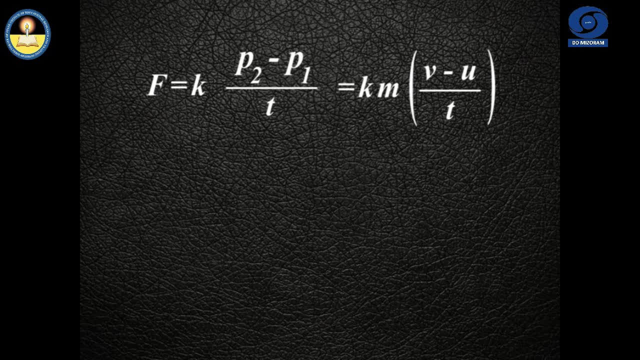 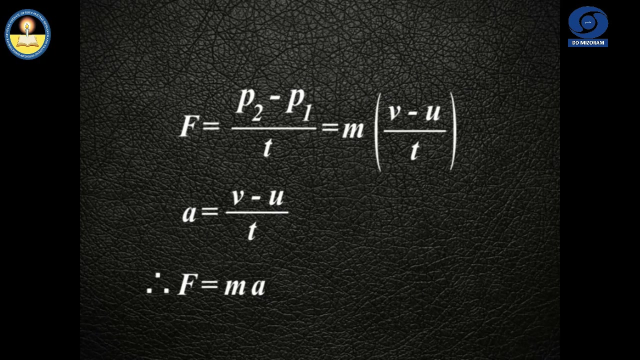 Since the value of proportionality Constant is unity, so the applied force is equal to the rate of change in momentum. In other words, force is equal to the product of mass and rate of change in velocity. We know that the acceleration is equal to the time rate of change of velocity. 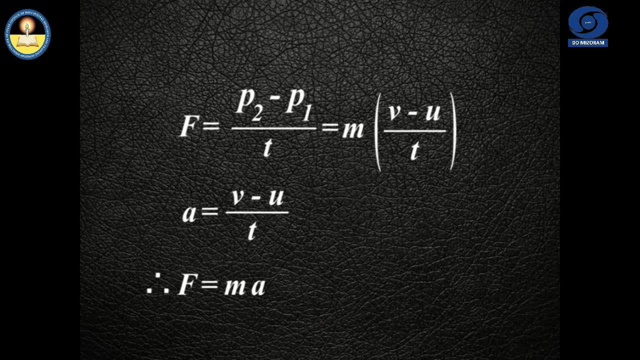 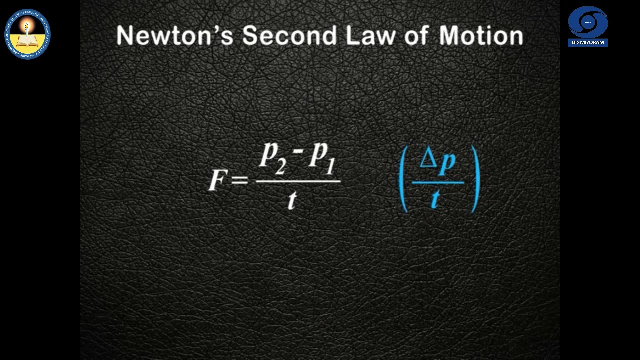 Therefore, force is equal to the product of the mass and the acceleration. This is the commonly known form of Newton's second law of motion, According to which the applied external force is equal to the time rate of change in linear momentum. See, it can be seen that small force. 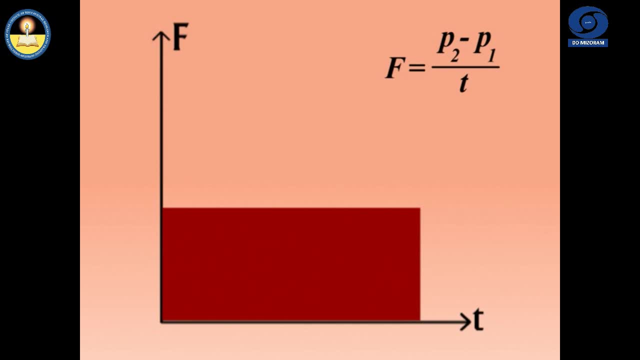 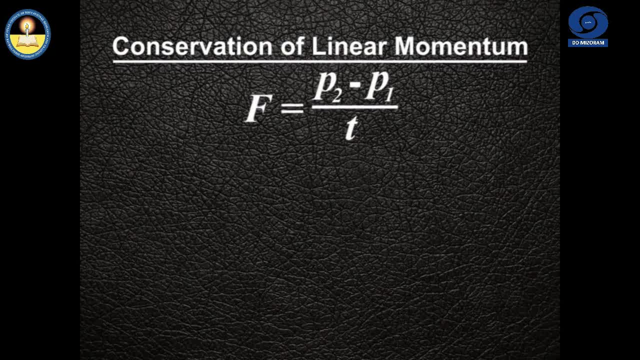 We know that the external force acting on a system is equal to the rate of change in momentum. It can be noticed: if the external force on the system is zero, the initial and final momentum comes out to be the same, Since the momentum is a vector quantity. therefore, the linear momentum is equal to the rate of change in momentum. 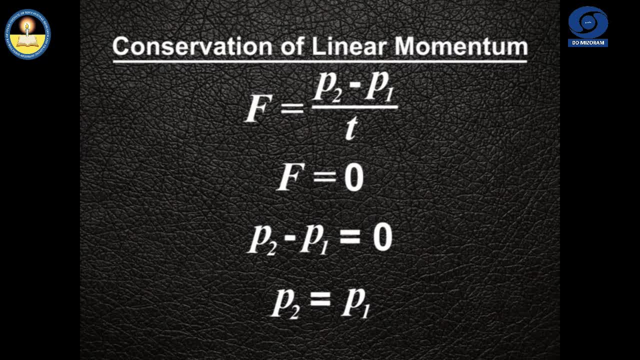 Since the momentum on the system is equal to 0, the initial and final momentum also remain the same. We know that the internal force acting in power acts on the position and the z-axis on the system, Since the momentum is a vector quantity. therefore, the linear momentum comes out to a desired level. 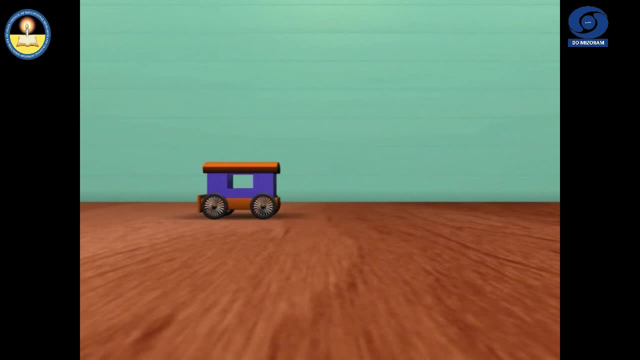 The horizontal force acting on the system is equal to the truth on a ruling of a designed system. These forces are oriented to minor außer internal force, and not have any percentage. Since the momentum of an object is equal to, It is well established that when a collision occurs between two objects, 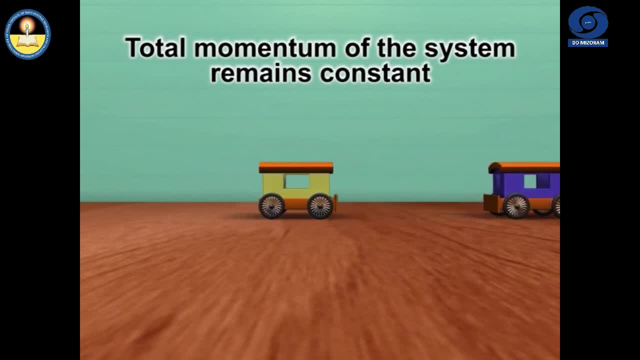 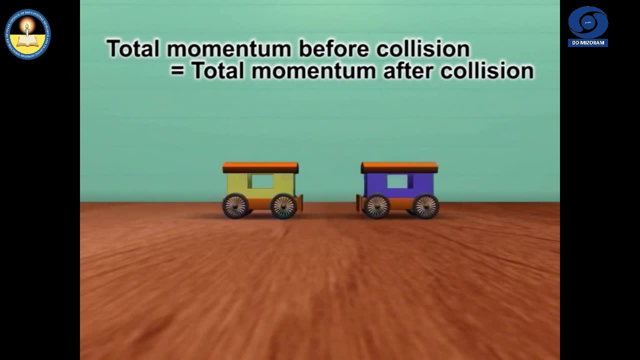 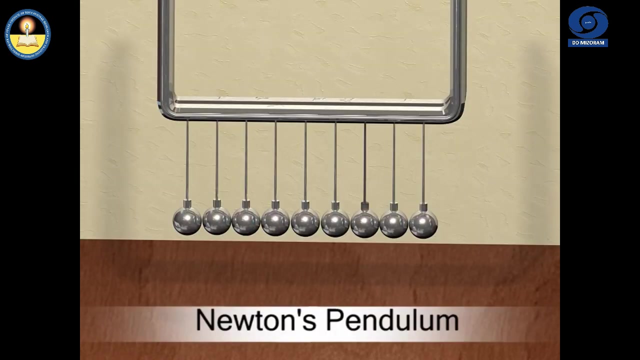 total momentum of both the objects remains constant. That is, the total momentum of the two objects before the collision is equal to the total momentum of the two objects after the collision. Let us look at an activity using Newton's pendulum. It consists of a series of identical metal balls of the same size. 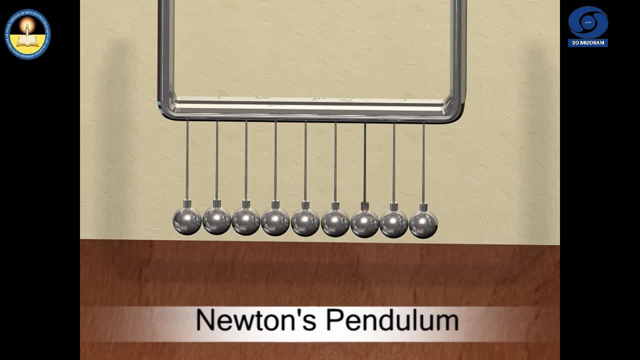 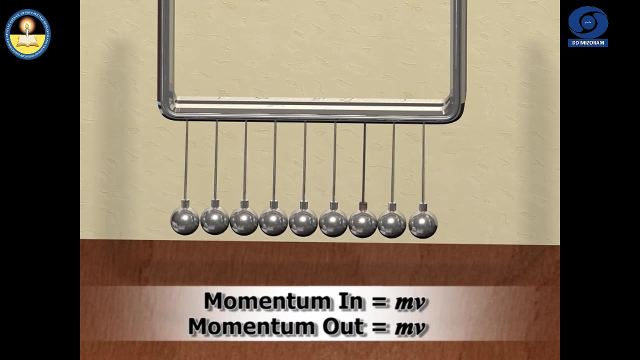 and all the balls are suspended on a metal frame in such a way that they are just touching each other when at rest. as shown, When one ball is pulled away and is allowed to fall, it strikes. It strikes the next ball of the series and comes to rest. 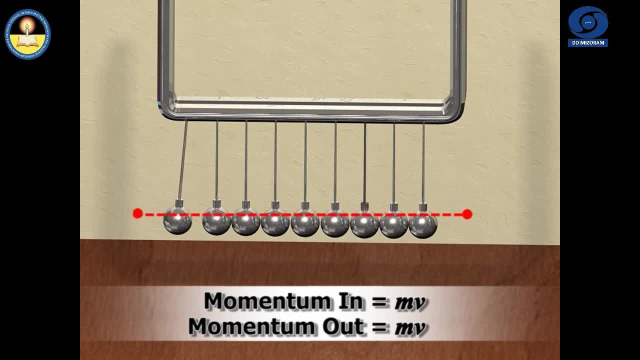 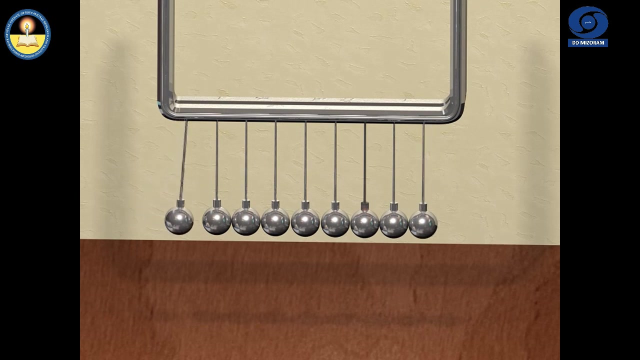 Whereas the last ball of the series acquires the same velocity and swings as high as the release height of the first ball. This shows that the balls simply exchange velocities. In other words, the final ball attains the momentum of the first ball. 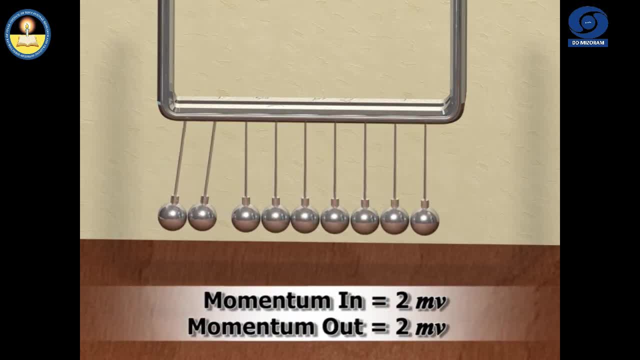 Let us repeat the activity by starting more than one ball in motion. as shown, It can be noticed that the same number of balls on the opposite side swing almost as high as the release height. Once again, the balls simply exchange velocities and the total momentum before the collision. 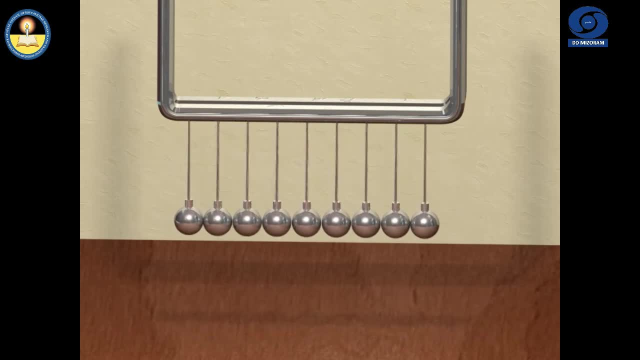 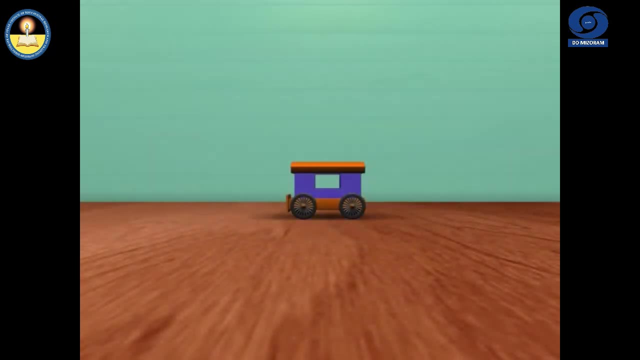 is the same as after the collision. Let us see some examples related to the law of conservation of momentum. Let us see a situation of an elastic collision, When a stationary trolley of mass m has a head-on collision with a moving trolley of. 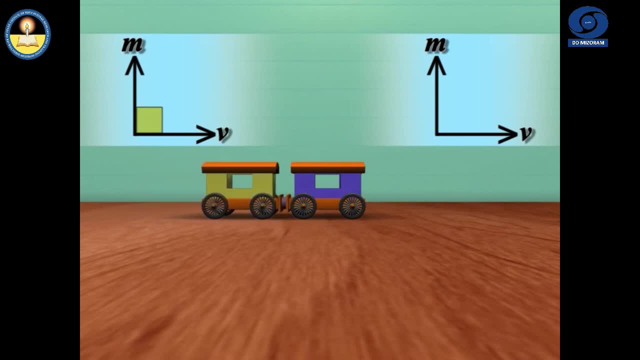 the same mass. then, after the collision, the first one starts moving and the second one starts moving. The second trolley of mass m starts moving with the velocity of the second trolley, while the second one comes to rest. That is, their velocity as well as their momentum are interchanged. 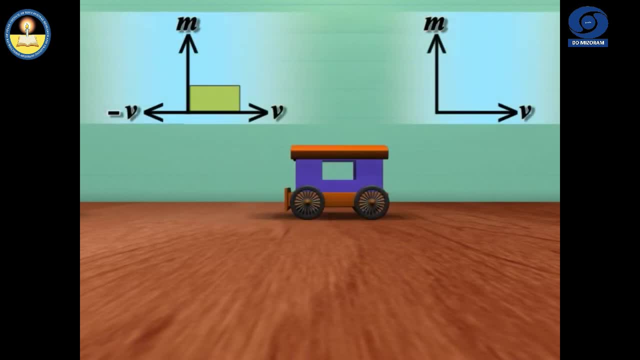 Further, if both the trolleys are of unequal masses, then after the collision the velocity of one trolley increases while that of the second decreases. Let us repeat the activity by starting more than one ball in motion, as shown. Let us look at the recall of another trolley of mass m and the total momentum of both the 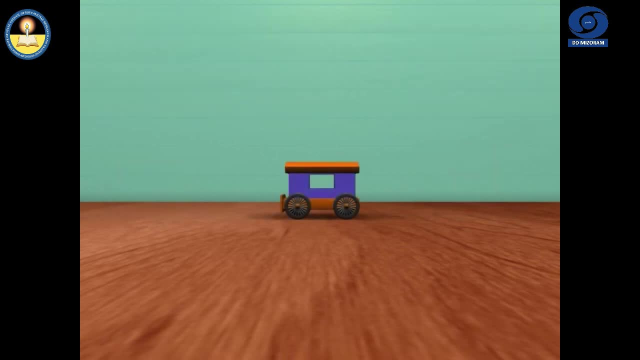 trolleys remains the same. Let us see a situation of an inelastic collision. When a stationary trolley of mass m has a head-on collision with a moving trolley of the same mass, then after the collision, both the trolleys move together with a velocity. 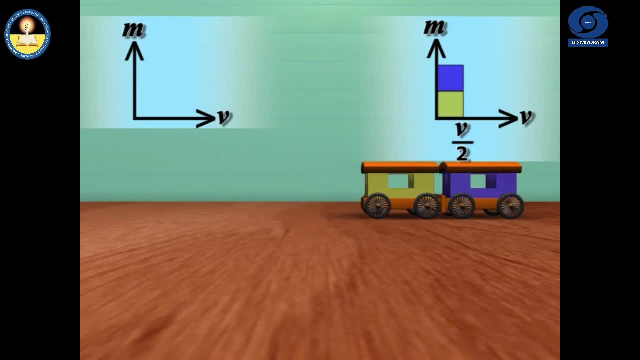 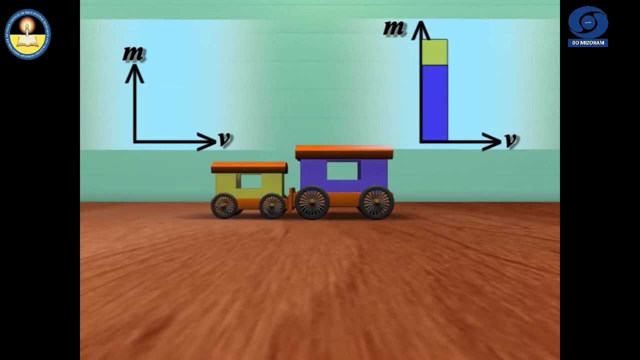 which is half of the velocity of the second one. Again, their momentum remains the same. Further, if both the trolleys are of unequal masses, then after the collision both the trolleys move together In such a way that the total momentum of both the trolleys remains constant. 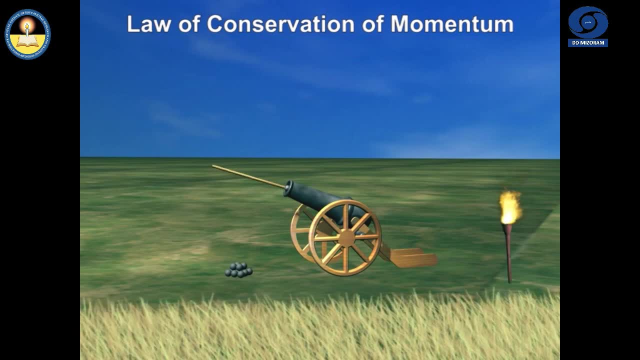 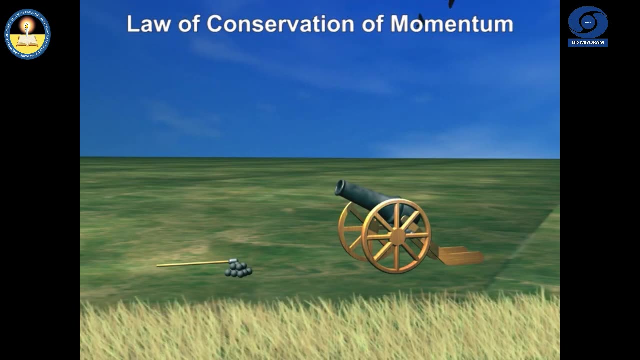 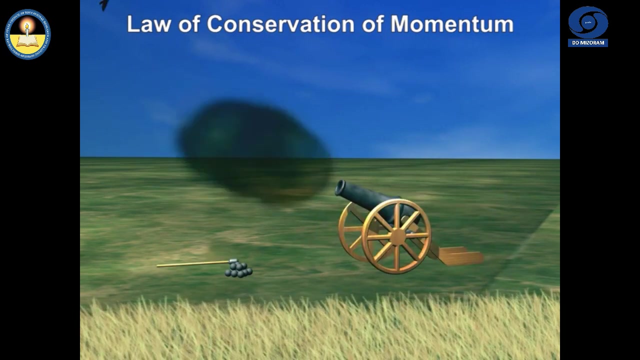 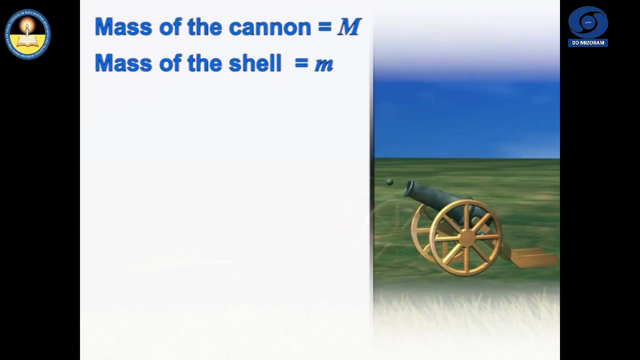 The coil of the cannon in opposite direction is also due to the conservation of momentum, Since the initial momentum of the system is zero. hence, the cannon has to move in the opposite direction to conserve the momentum, as can be seen, Since the initial momentum of the system is zero. 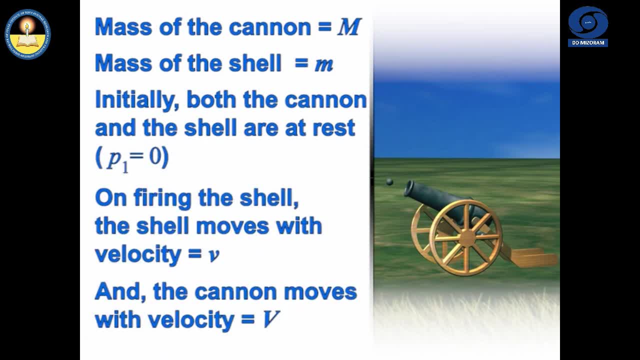 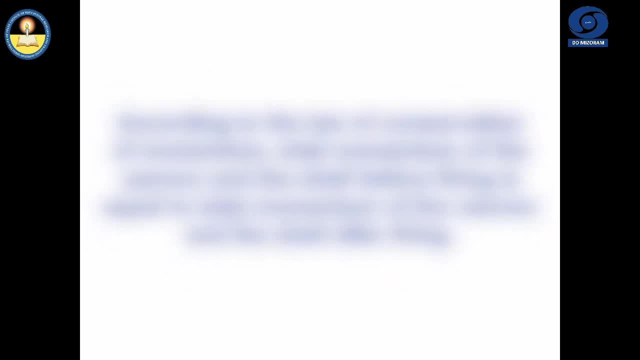 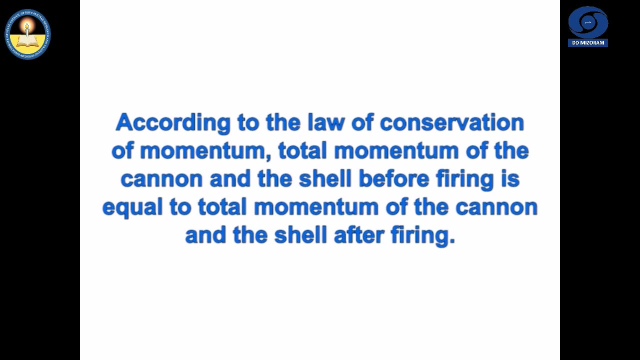 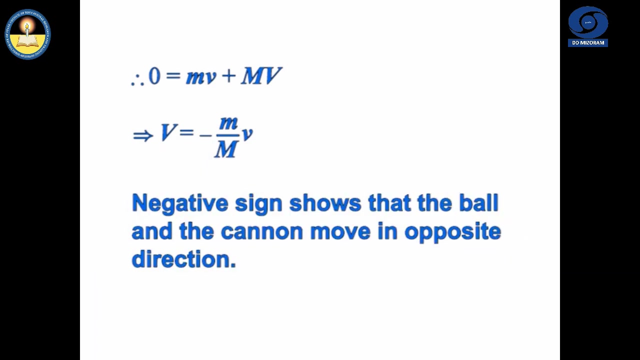 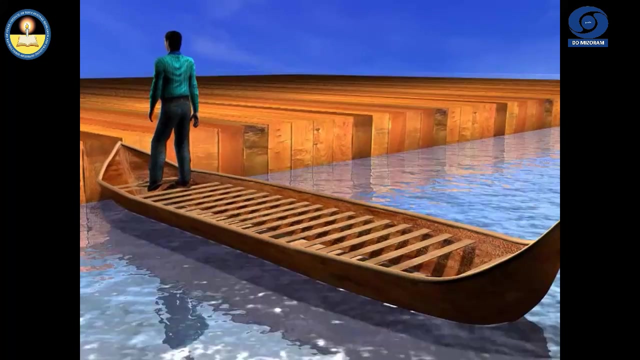 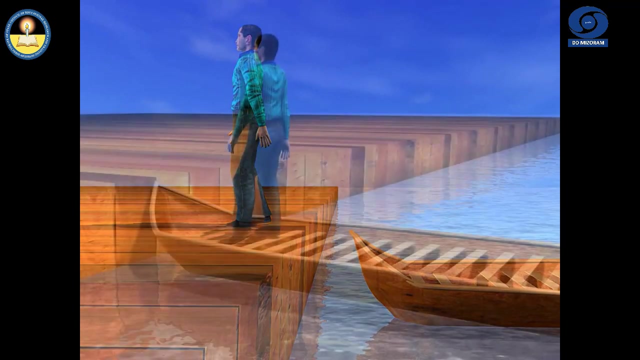 hence the cannon has to move in the opposite direction to conserve the momentum, as can be seen. Similarly, when a boy jumps out from a boat to the bank of a river, the boat slightly moves away from the bank because the inner part of the boat is moving away from the bank. 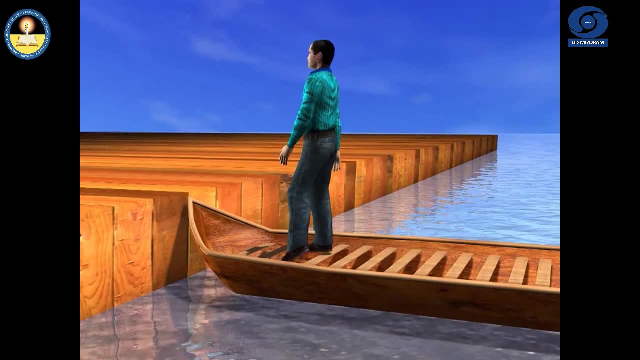 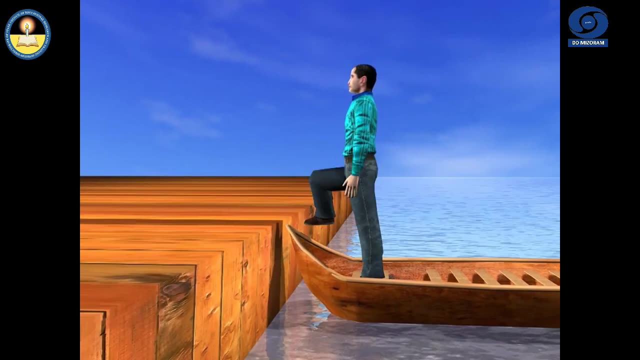 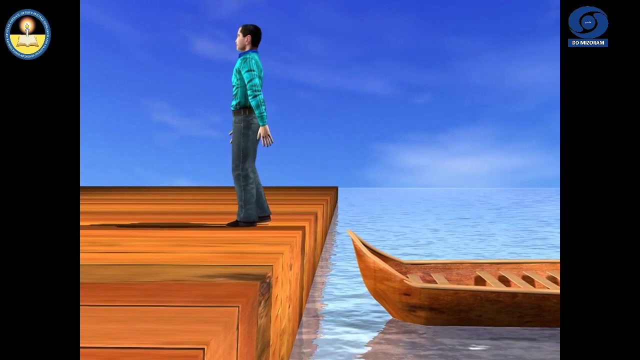 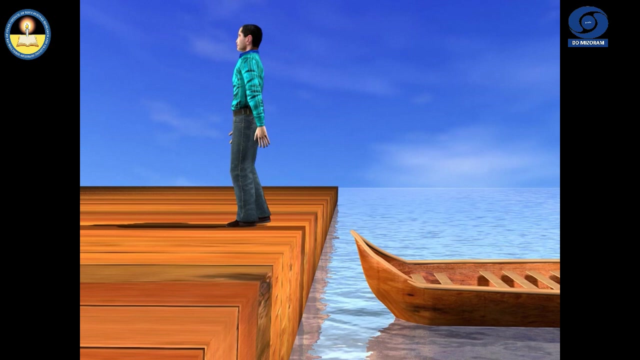 In the initial, total momentum of the boat and the boy is zero. When he jumps out from the boat to the bank, total momentum of the boy and the boat should also remain zero. This is possible only if the boat moves in the opposite direction.